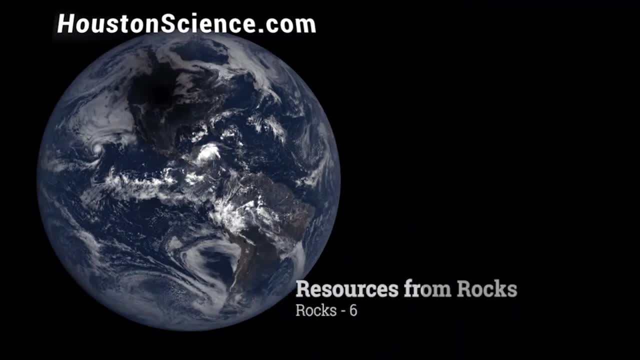 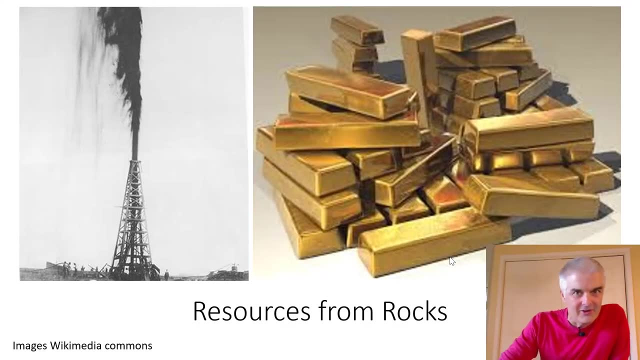 So probably the big question is: who cares about rocks? They're just stuff underneath the earth, right? No, because we can get cool stuff from the ground, Like you're probably all interested like gold. Where'd the gold come from? They've got to dig it out of the 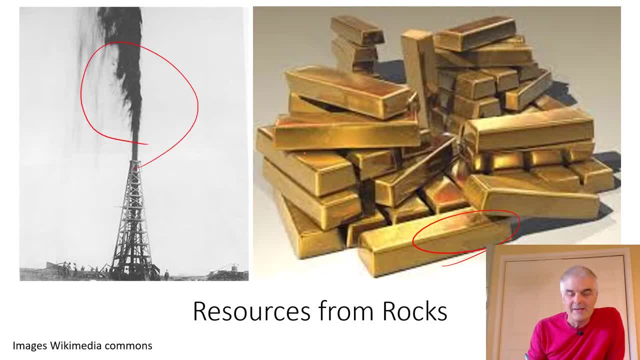 ground. Well, what about oil? This is one of the old oil gushers from way back when. Those are valuable things for the world, right? Minerals and rocks. where do you get them from, and how do you find them? That's so interesting. Well, it turns out that there's. 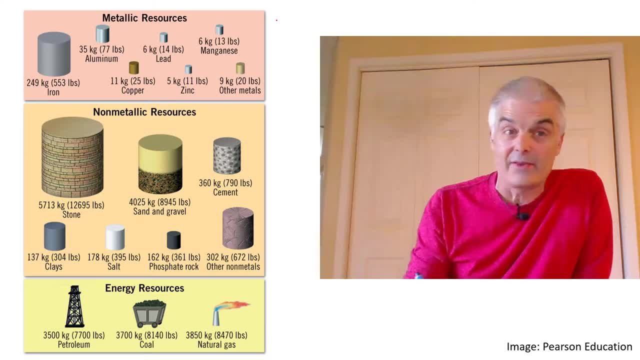 three categories of resources that we want to get out of the ground. There's metallic resources, some type of metal- iron, aluminum, copper, zinc, gold, magnesium, lead, all that cool stuff, right- Or non-metallic- Now, these are just like the rocks, by the way, guys. 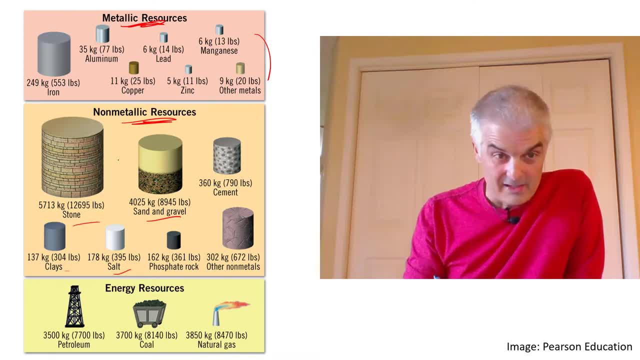 Cement, sand, gravel, salt, clay, stone. We make our buildings out of these things, So these are just rocks, but they're useful and valuable, right, Depending on what you're doing, particularly if you're building things. And then we've got energy resources. We're 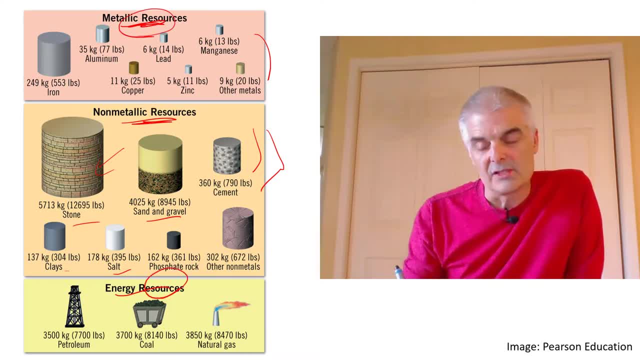 going to get into that in a minute. We're going to just focus frankly on number one and number three, if you will, as we talk about how do you find it? So it comes back to the geology, the underlying geology of 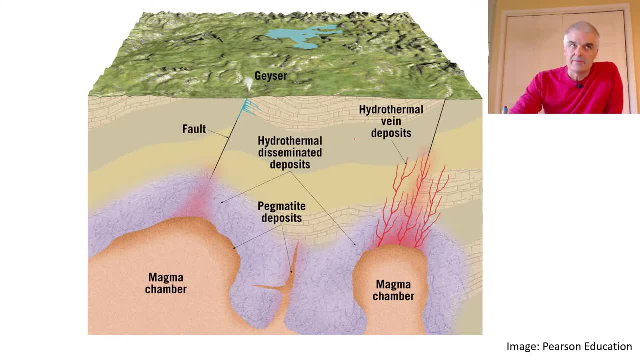 the area. So let's talk about the metallic resources. The metallic resources are not all like, spread all over the earth. They're in certain pockets. You've known this. You've studied history. You've talked about the gold rush of the 1849 near San Francisco. There's 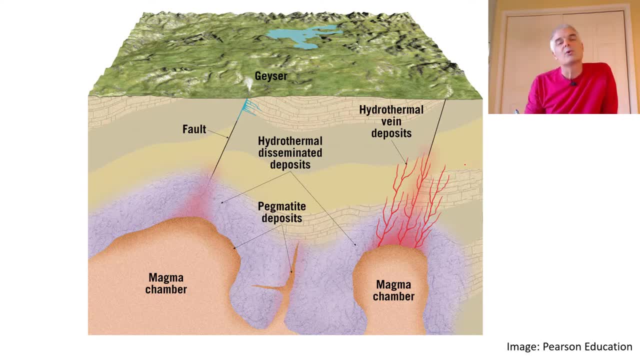 all these big gold rushes and they went to a certain place in the world. Why did they go to a certain place in the world? Why did they go to a certain place in the world? Why did they go to a certain place in the world? Because something happened geologically: a. 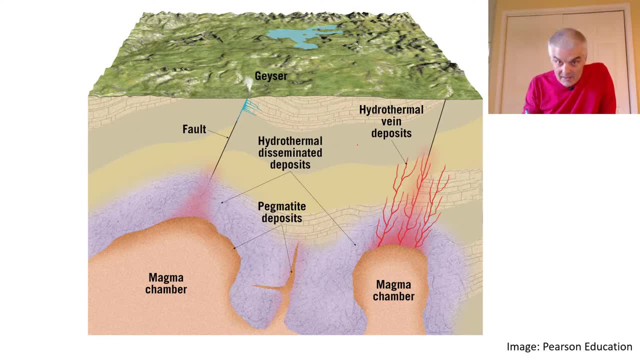 long time ago and it's almost always had to do with water. Look at this word: hydrothermal vein deposits. Hydro means water, Thermal means heat, So hot water. So the magma chamber gets somehow gets some water in it, And water you ever like. pour water on something that's. 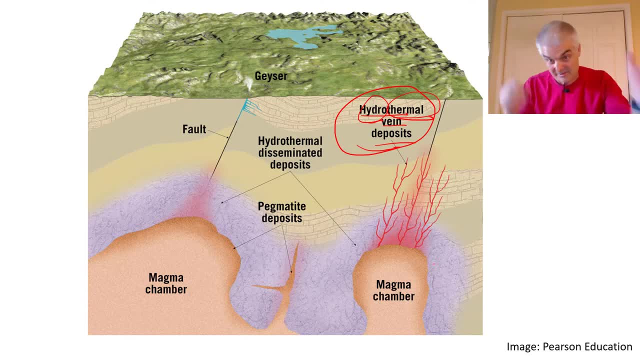 super hot, It just instantly boils. This is like magma: super hot, liquid, cold hot stuff, right. It's not cold. Liquid hot stuff, right. And what happens is is it shoots up the- I don't know these lines, if you will, these veins. And these veins can often, because the 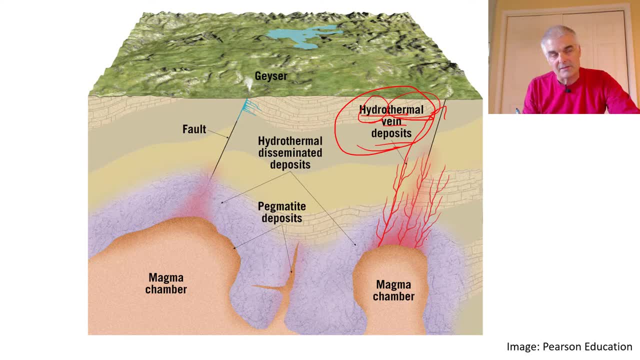 water somehow. I'm not sure I don't understand the chemistry of it, but the water somehow attracts particularly some of the more the higher density metals, the gold and such like that. And then what happens is the gold, or whatever these minerals are, tend to follow. 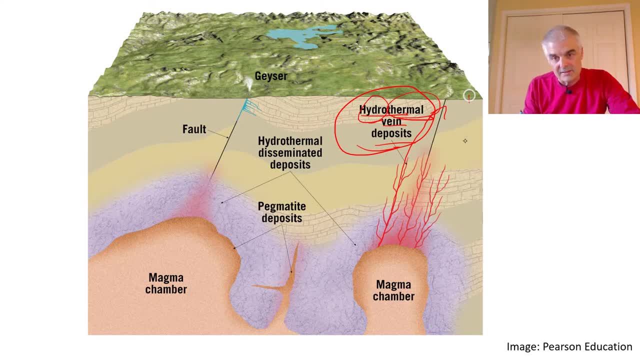 these veins, And so you know what the miner's trying to do is: he's trying to dig down, hello, trying to dig down a tunnel, and then tap into that vein and boom, rich guy right. So you can't see it really well, but you can tell that it's very, very rich. 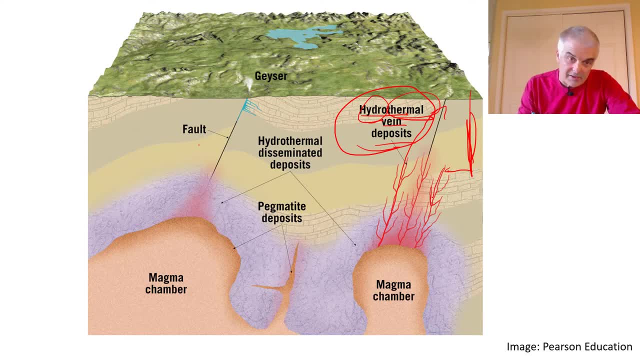 Yeah, that's pretty interesting, right. So there's it. often these happen to do with hydrothermal. Now, sometimes it's caused by a fault. Again, we'll learn about faults- Earthquakes that's kind of a thing- But the faults sometimes create a way for the water. 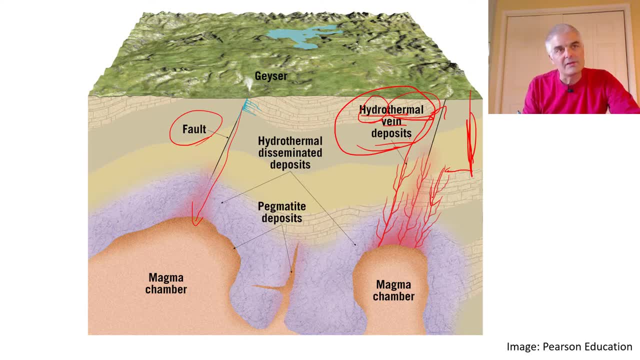 to get down that creates these types of deposits. So I mean, long and short of this is that geologists are looking for places like this, and when they find them, then of course they find a place that's worth digging and then bing. maybe they find something, maybe they. 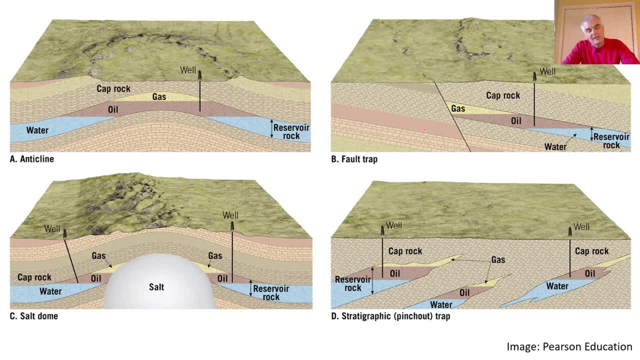 don't, But when they do, they find something, or they predict that something might be in can become rich. Now let's talk about, though, the natural gas, oil, this kind of stuff. What about the energy resources? Well, it turns out that energy resources always come from sedimentary. 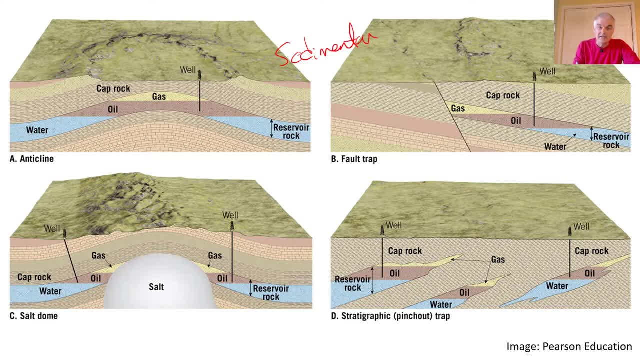 rocks. You know the history of Texas, of course, has a whole lot to do with sedimentary rocks and oil. right, What made Texas wealthy was discovering oil, because Texas is filled with, like thousands and thousands of feet of sedimentary rocks And it turns out that, and remember oil, if you will- 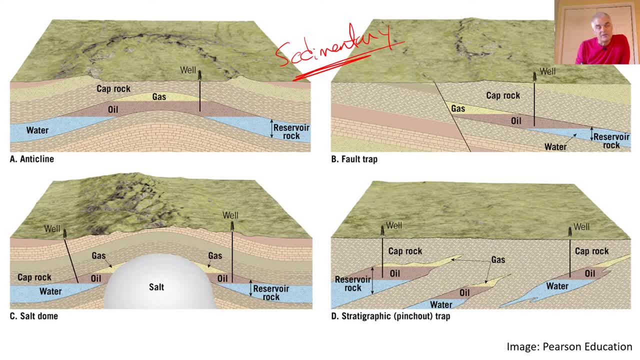 or the coal- same kind of idea. it comes from dead creatures And the dead creatures then get trapped under the ground and then they find places. But you need to find places where it's easy to get access And it turns out they often will be in kind of this shape and it gets caught. 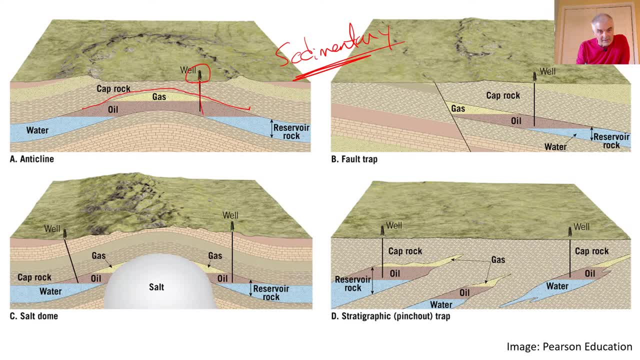 And what you do is: you like drill wells- This is one of those classic wells- And you want to find a place where you can drill a well. And you want to find a place where you can drill a well. You can. it's trapped, So this is the reservoir rock, So it's like the oil is sort of here, but 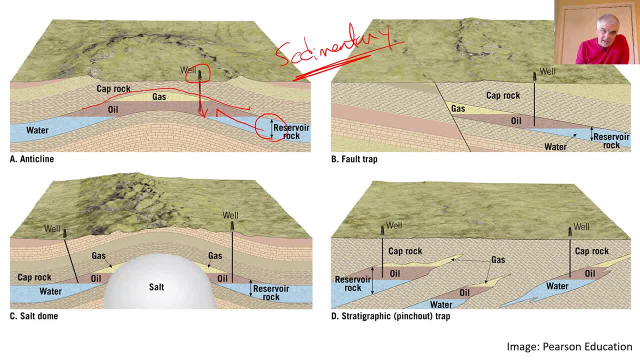 since oil is less dense than rock, it rises to the top and it gets caught in these domes, And then you just you punch a hole in it and then you get it out. It's really not that hard, This is.